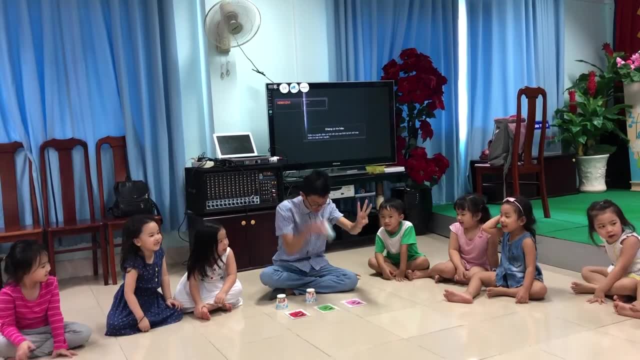 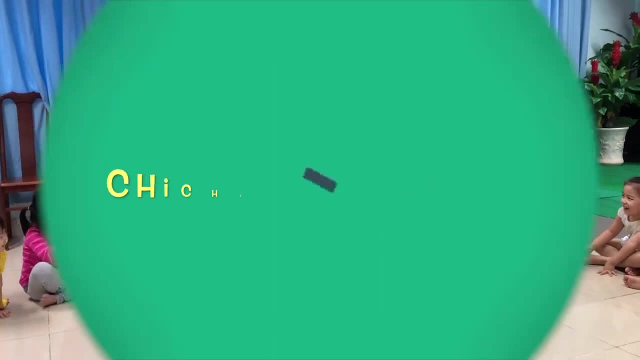 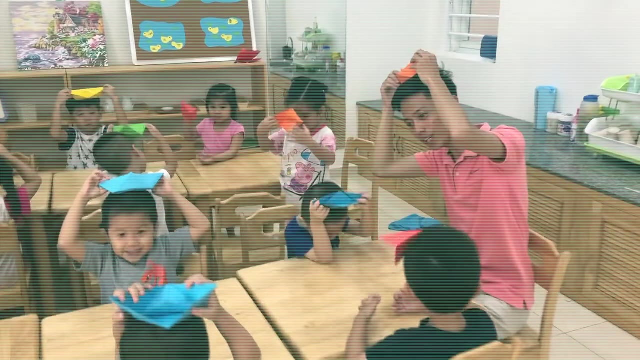 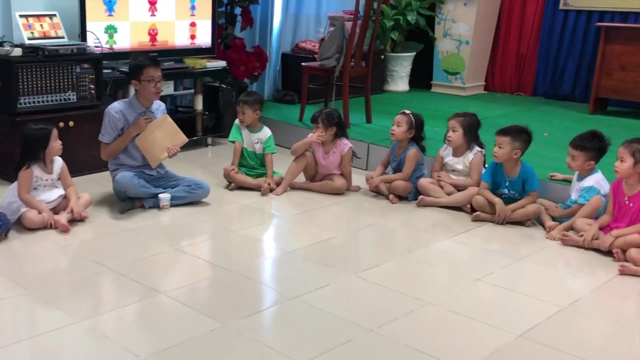 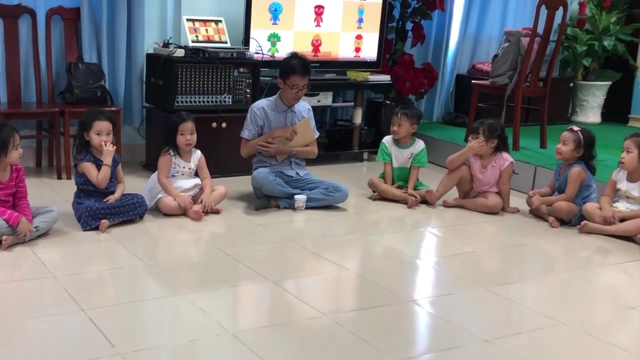 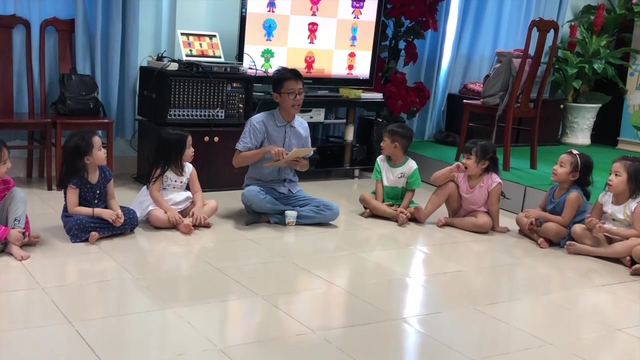 One, two, three, four. Oh no, Do you know colors? Yeah, Do you know colors? Yeah, Really, I cannot, I cannot open. You say: open, Open Again one, two, three, go. 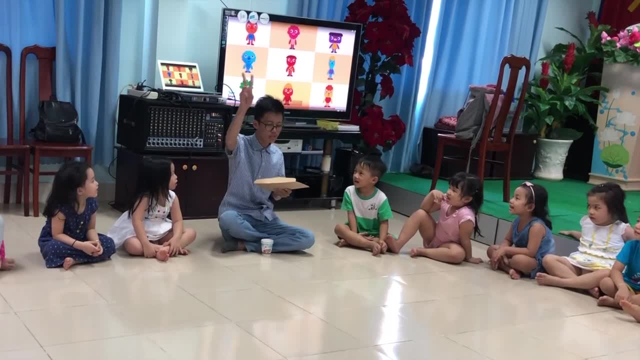 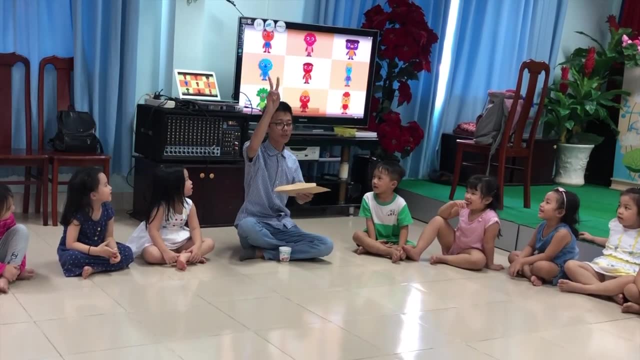 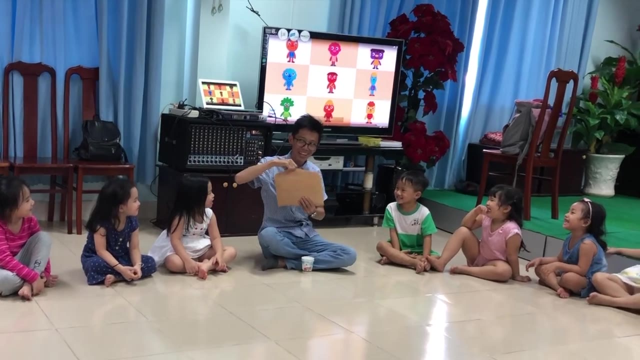 Open Open Again. one, two, three go Open Again. one, two, three go Open Again. one, two, three go Open. Oh, Open Again. the color is very. 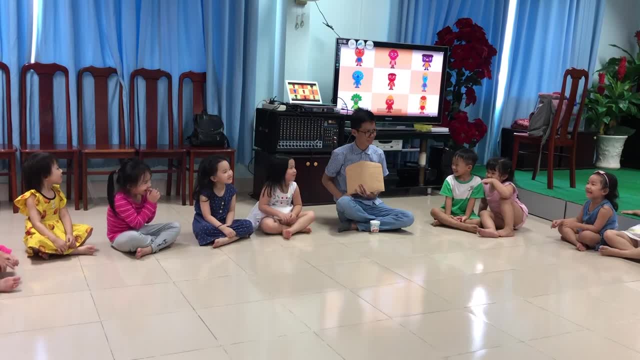 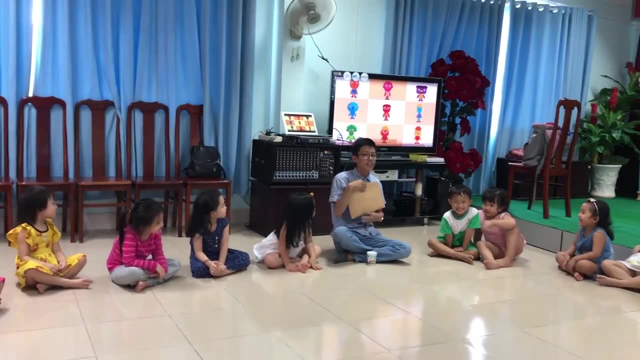 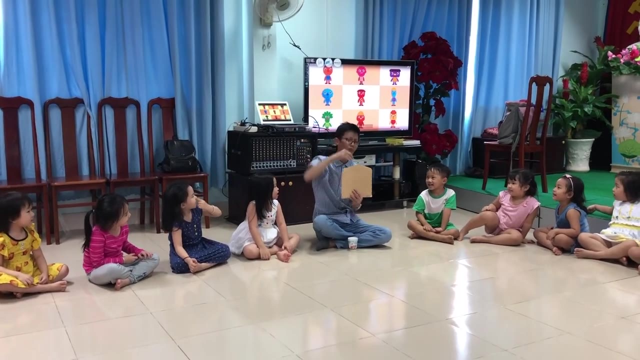 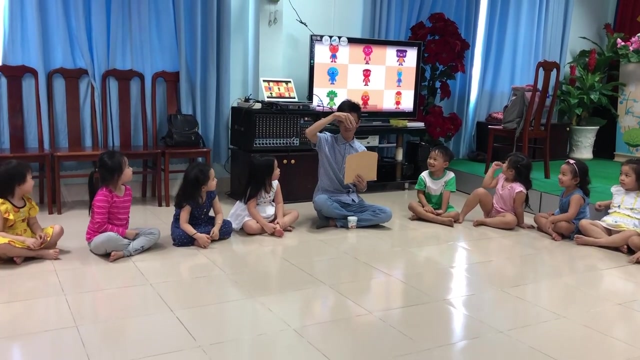 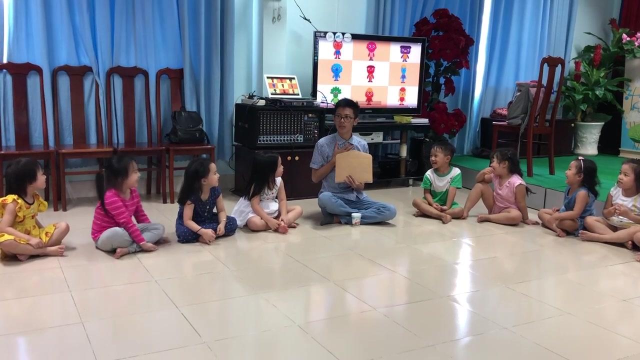 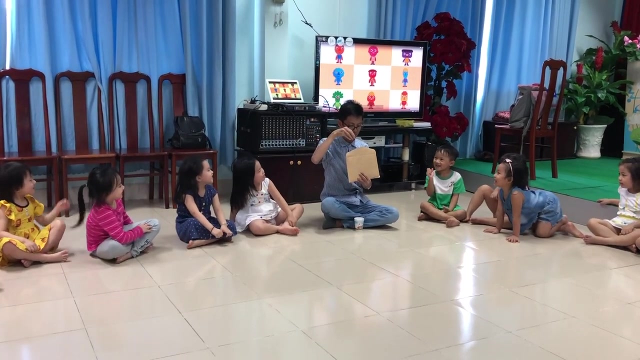 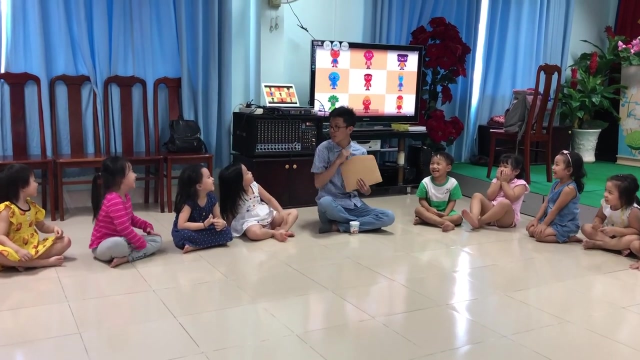 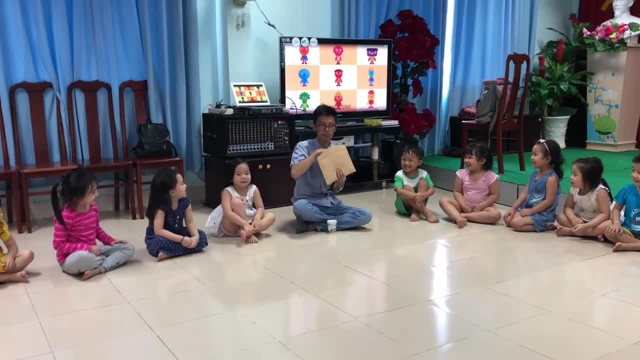 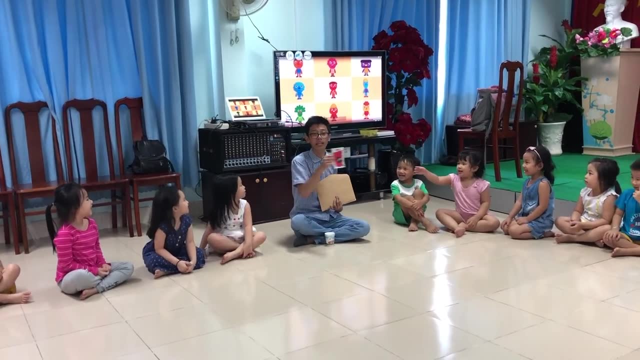 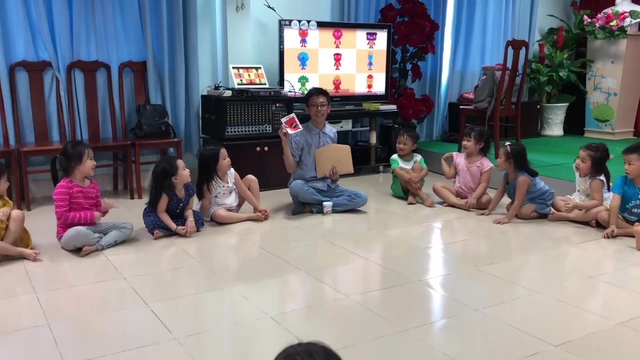 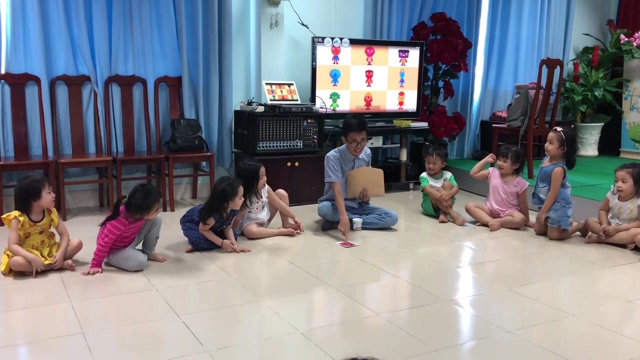 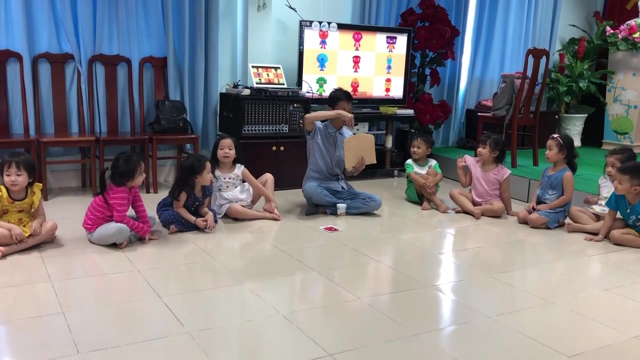 Go teacher, Go teacher. What color is it Again Red? It's red, It's red, It's red. What color is it? It's red, It's red. Properly Again. Go teacher, Go teacher. 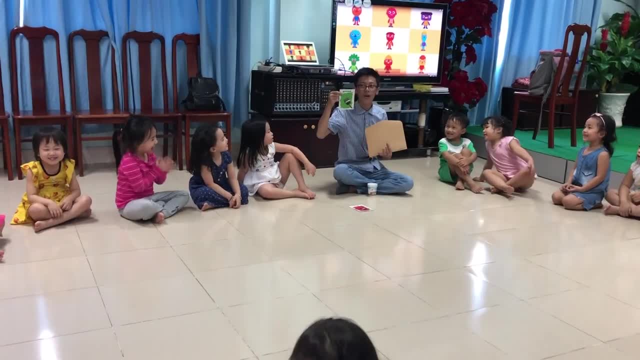 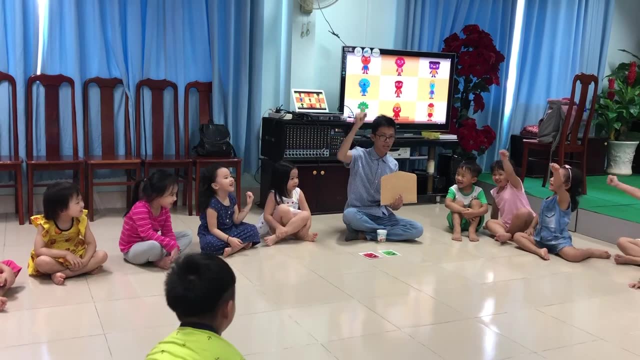 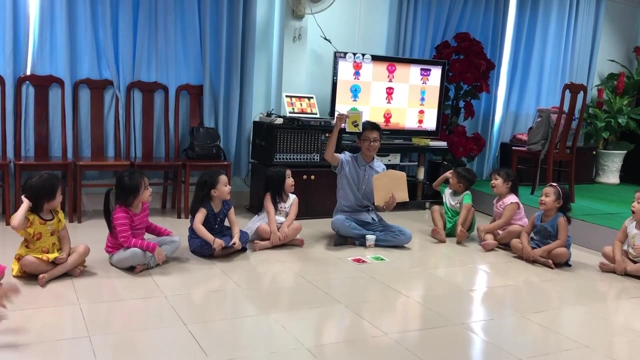 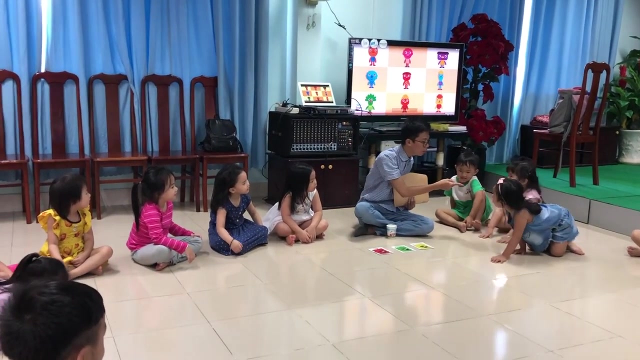 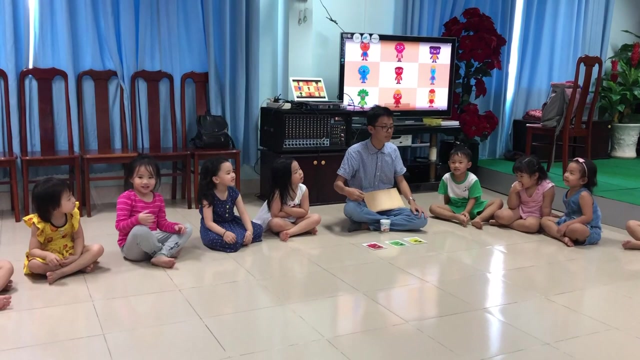 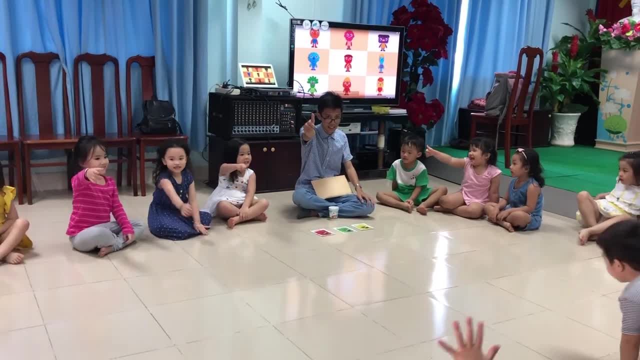 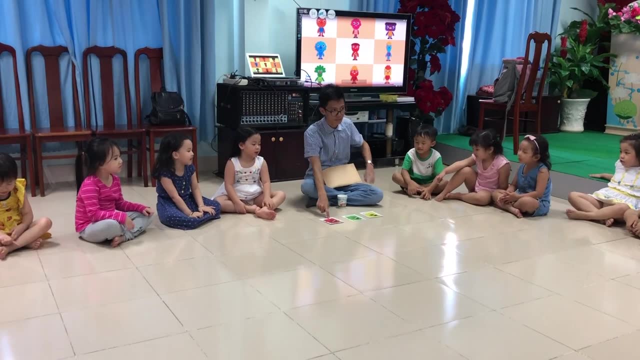 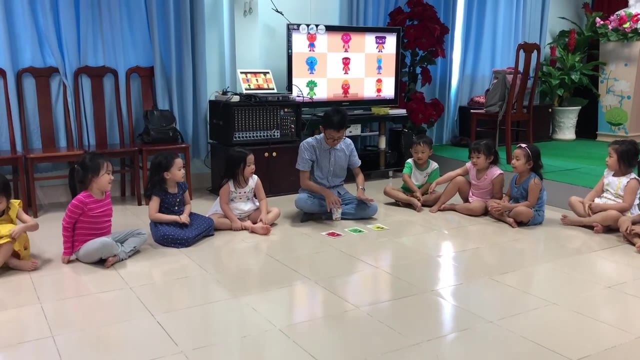 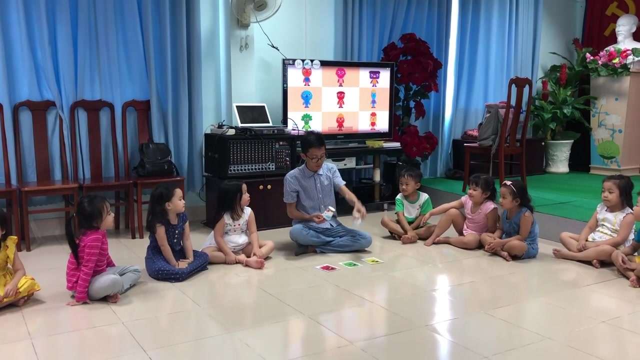 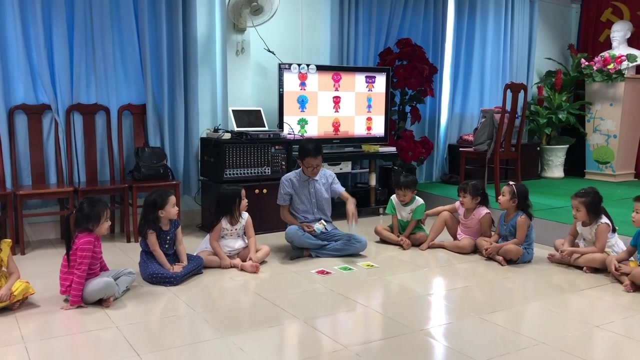 Alright, Ready, Ready, Ready. It's red, It's red, It's green, It's yellow, It's yellow. What's this? Go Go, One, Again, One, Again, Again, Again, Again, Three. 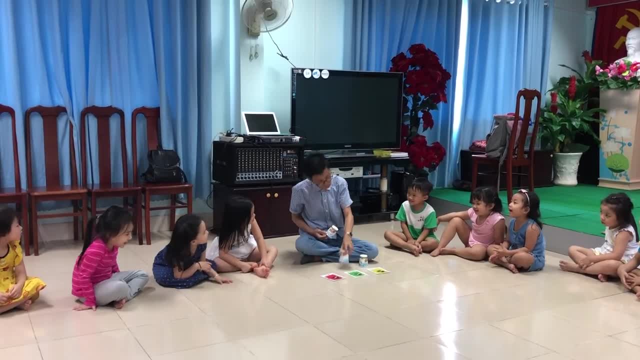 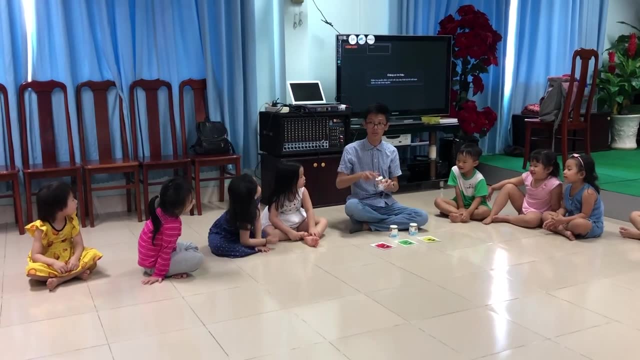 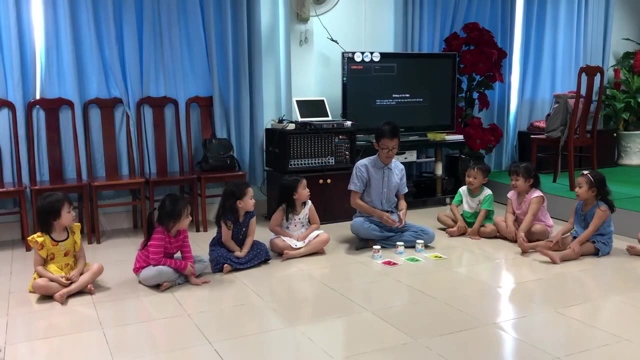 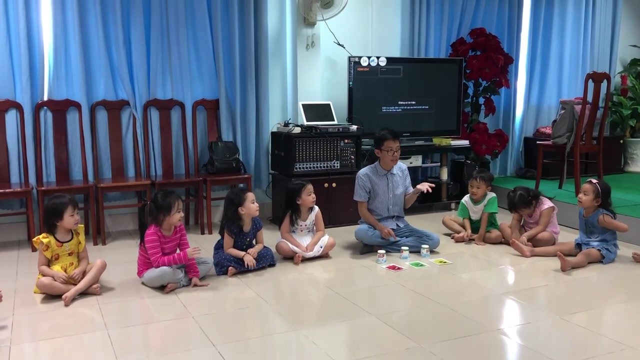 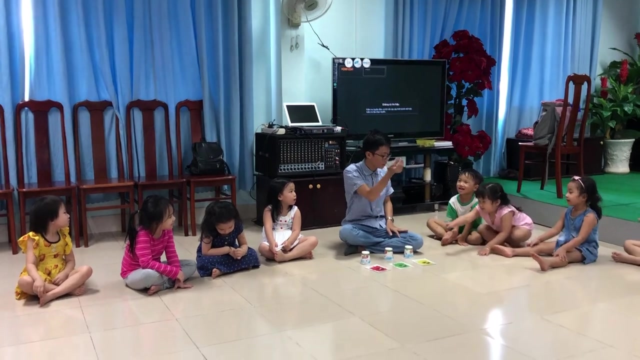 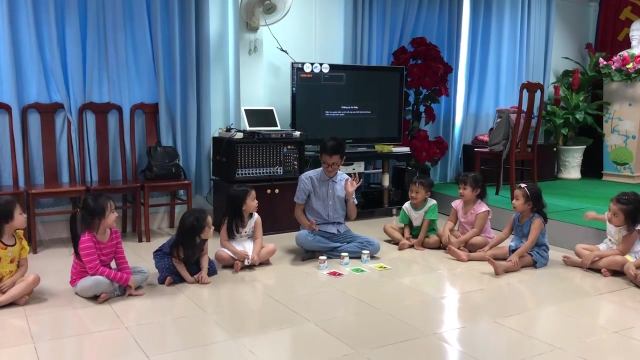 Two, Two, Three, Two, Two, Two, Three, Three cups, Three cups. One, Two, Three cups, Three cups, Three cups, And I have one marble. I will put the marble inside. Where's the marble? 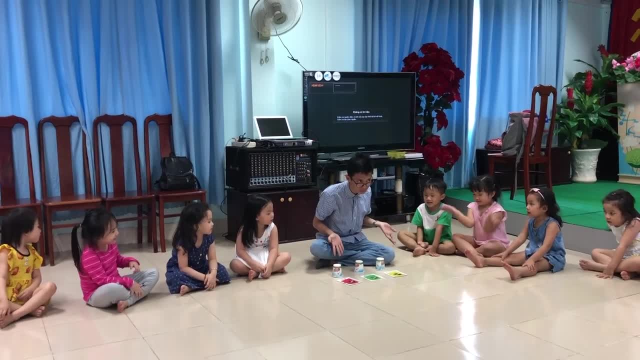 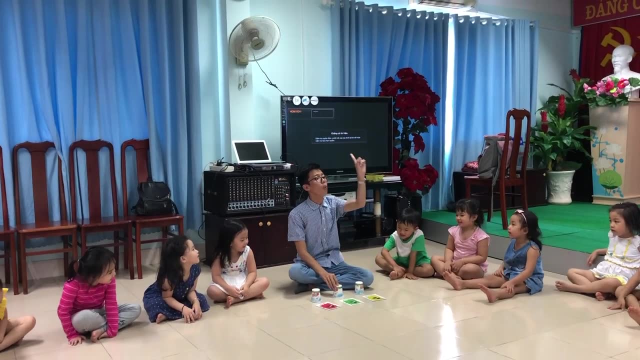 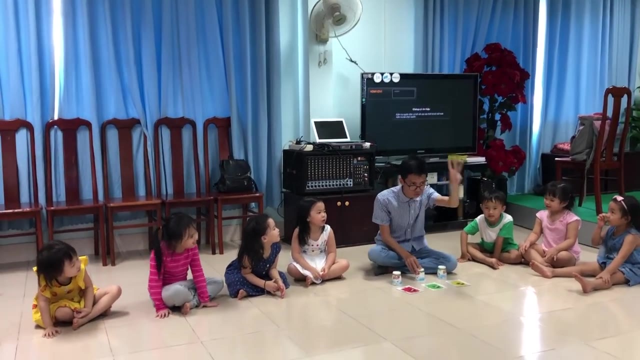 It's red, it's green or it's yellow, It's green, It's green. Very good, Say it's green, It's green. Can you count One? I can hear. I can hear One, Two, Three. 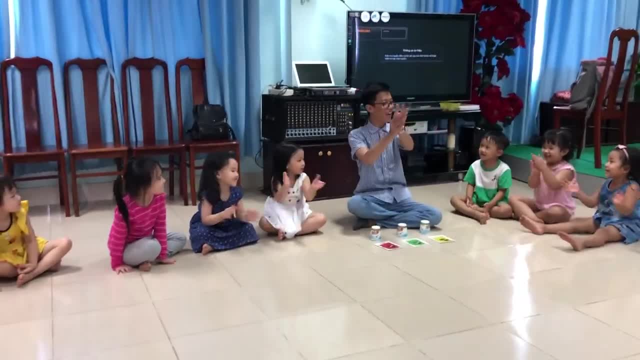 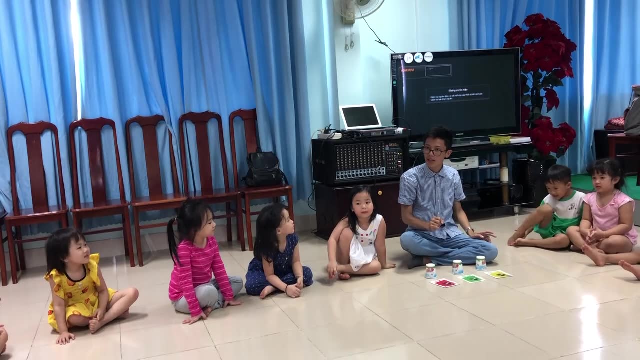 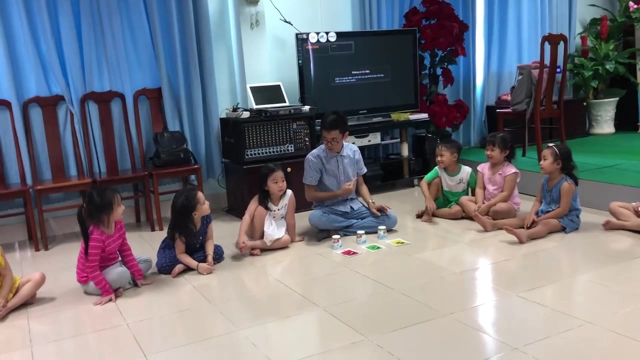 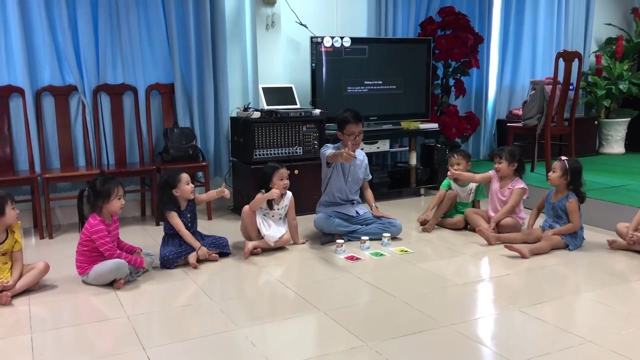 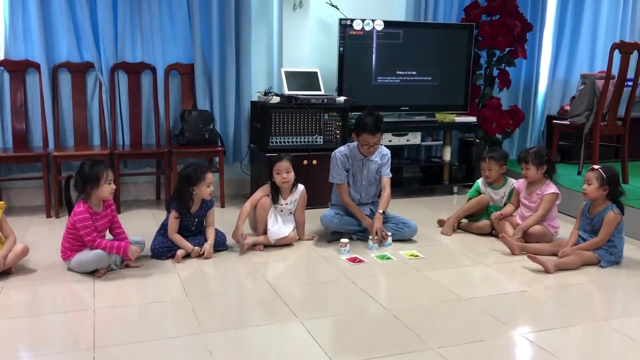 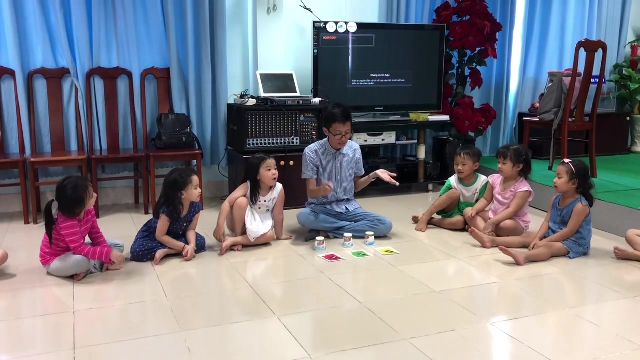 Up Say it's green, It's green, Ready. You have to watch carefully. You look Ready, Ready. Yes, I'm ready, Yes, Ready. Where One? It's yellow, It's yellow, It's red. 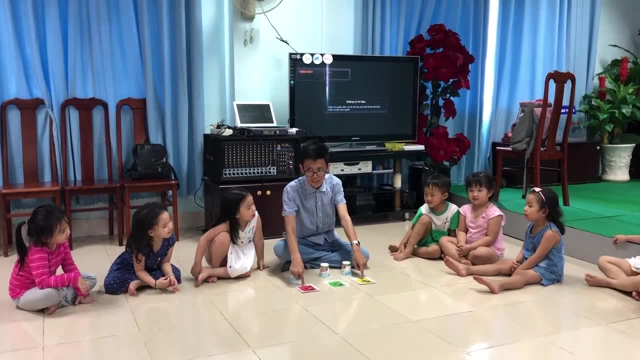 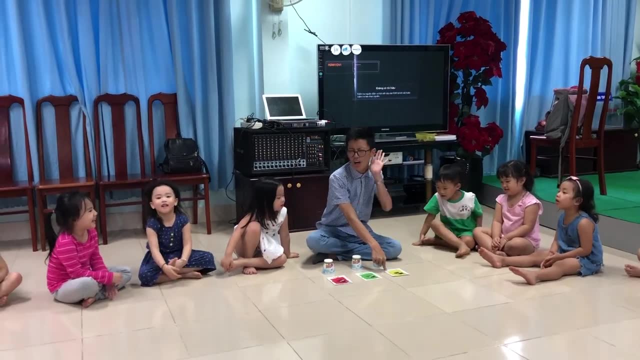 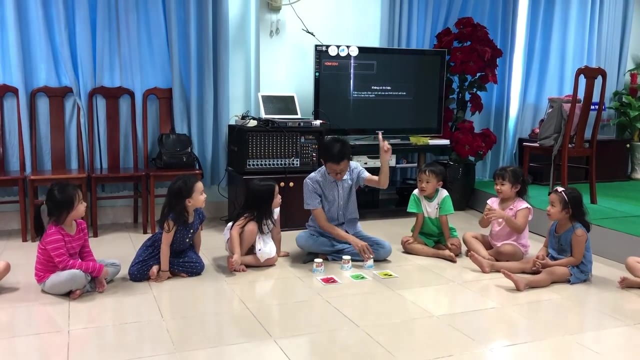 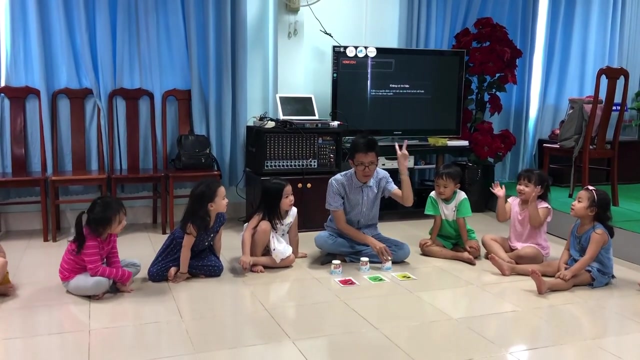 It's green, Yellow, Yellow Say it's yellow, It's yellow, It's yellow. I can hear It's yellow. Let's count One. One One, Two, Three. I can hear One, Two, Three. 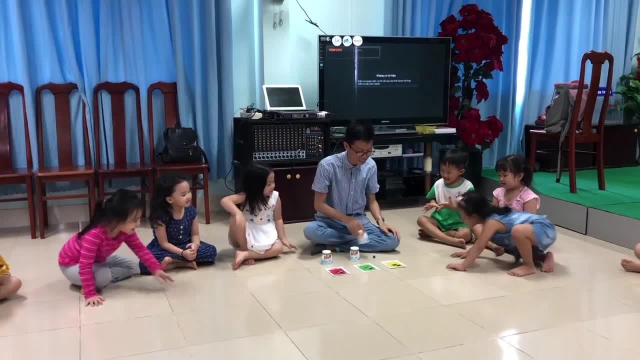 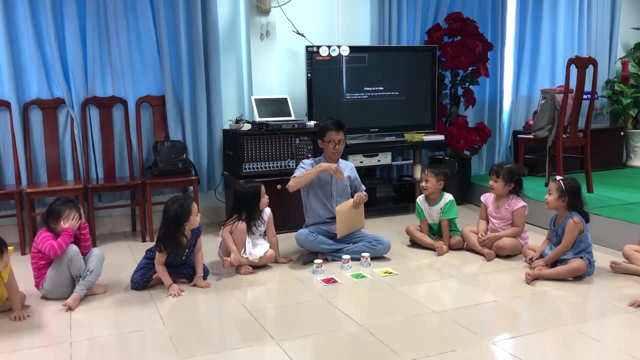 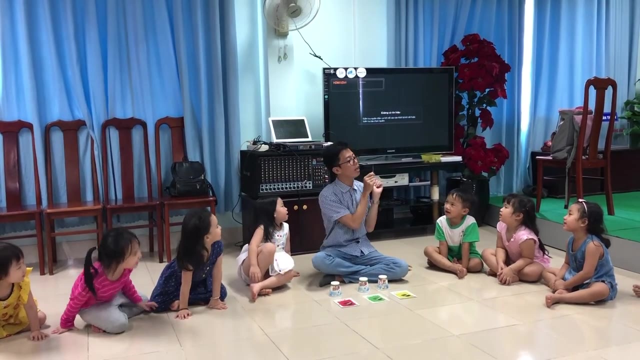 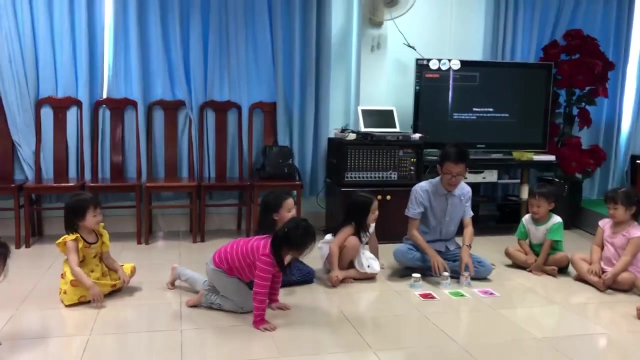 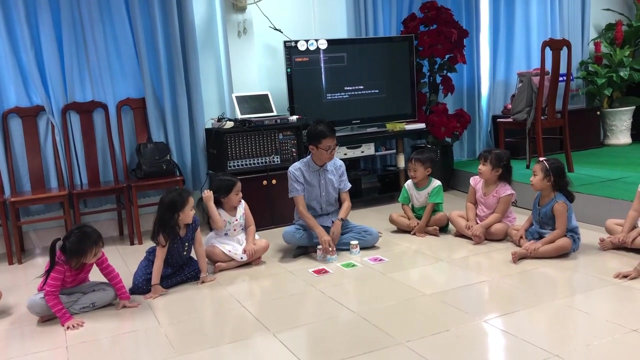 Wow Say: it's green, It's yellow, It's yellow, Okay, Okay, Wow, Pink, One more: It's pink, It's green. Oh, look, There's a bird. It's a bird. Oh, there's a dog. 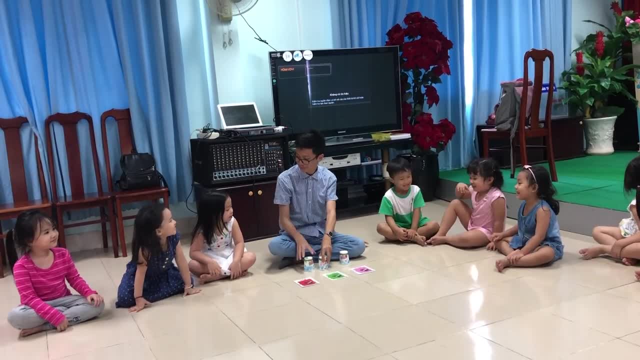 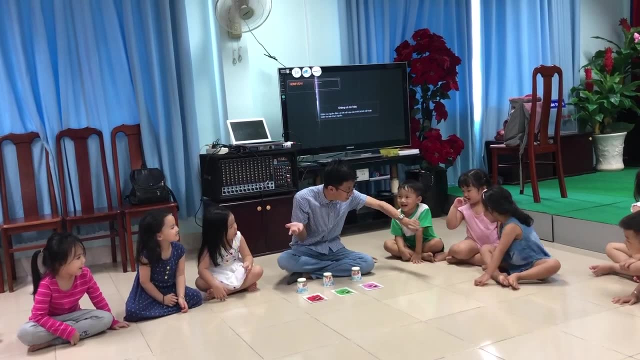 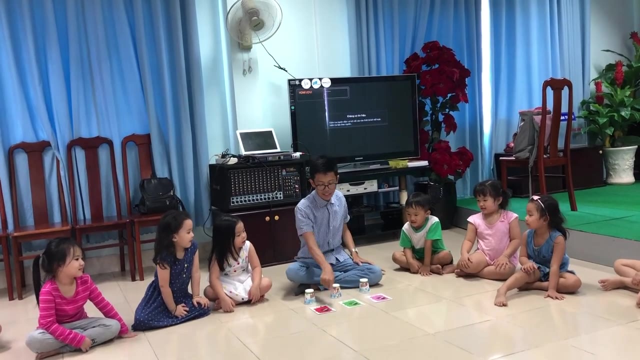 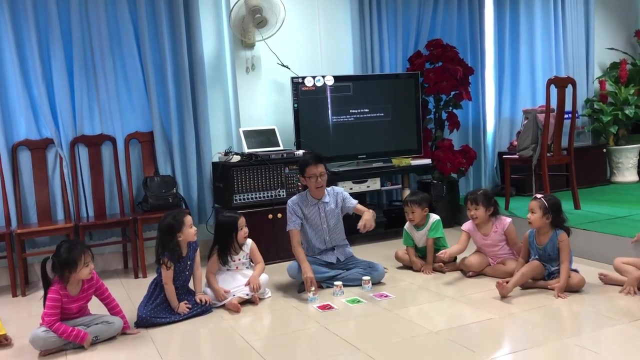 Oh, there's a dog. Where is the marble? Where is the marble? Sit properly, It's red, it's green or it's pink Red. Say it's red, It's red, It's red One. 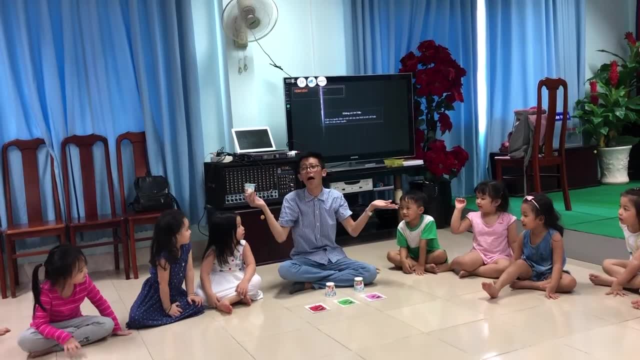 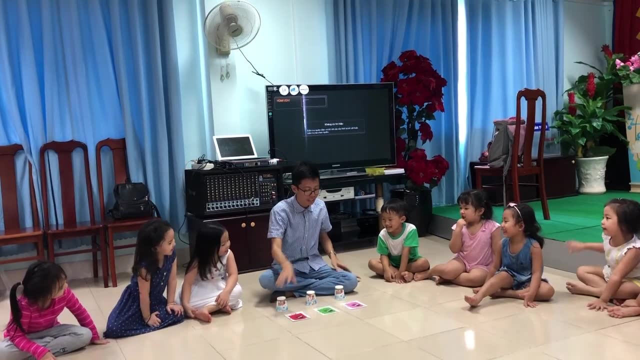 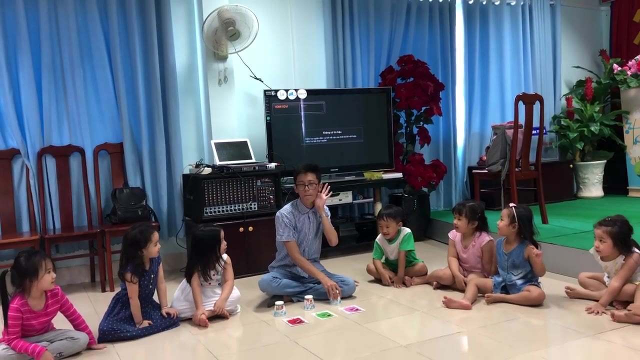 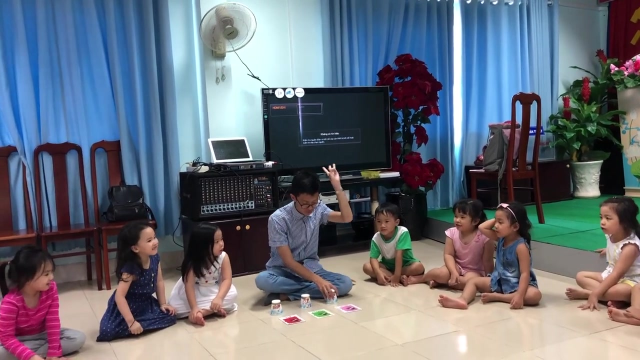 One, Two, Three, Four. Oh no, Not red, Not red, It's green. or it's pink, Pink Say it's pink, It's pink, It's pink. One, One, Two, Three. One, Two, Three. 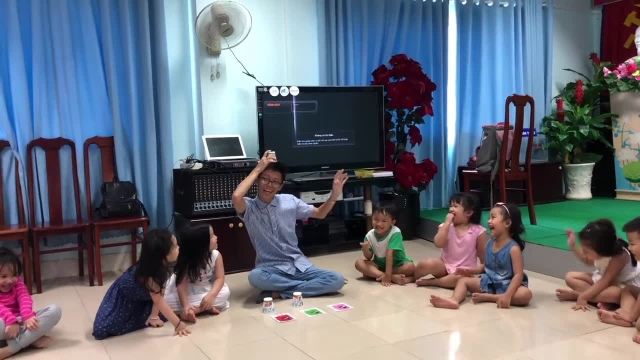 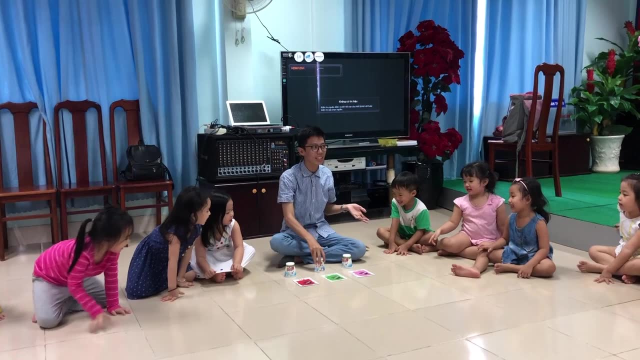 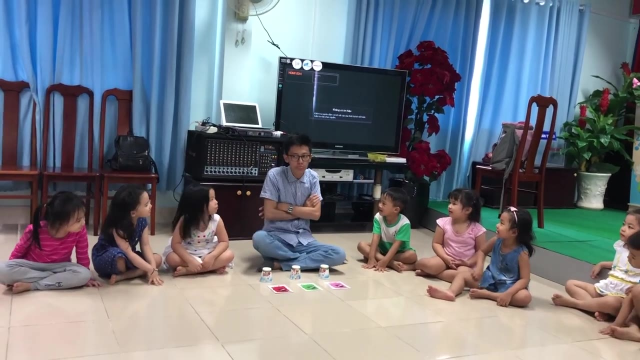 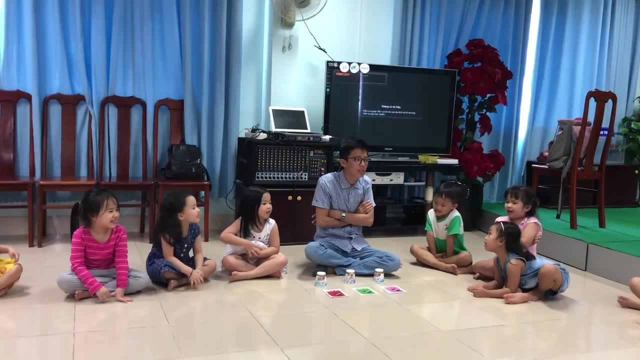 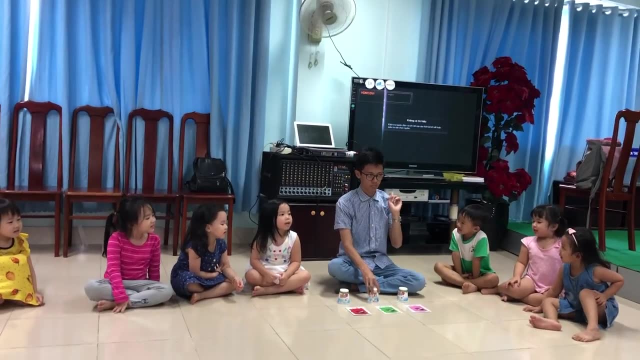 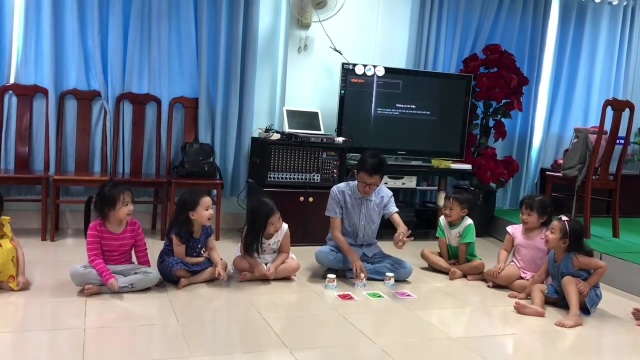 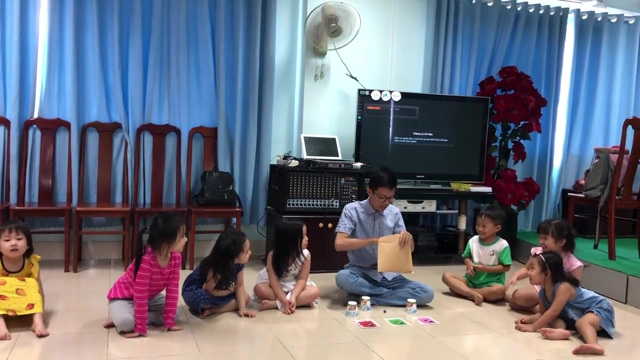 Sorry teacher, Sorry teacher, Sorry teacher. Alright, let's count. Say it's green, It's green, It's green. One, One, Two, Three, Yay, What color is it Blue? It's blue. 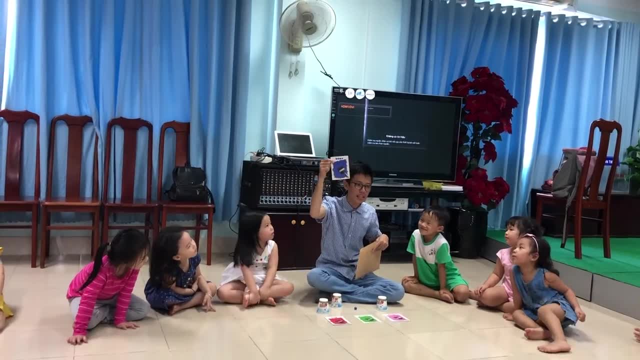 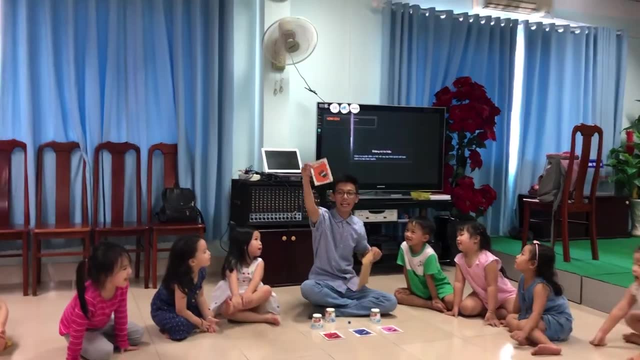 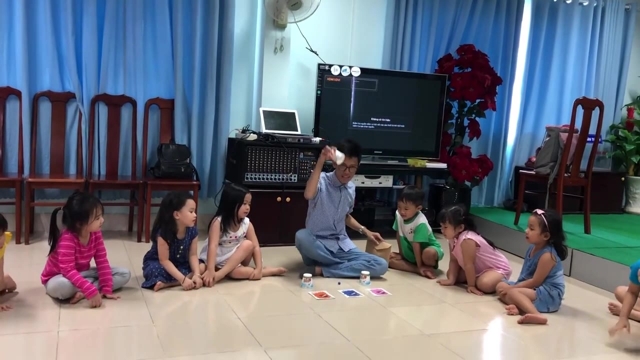 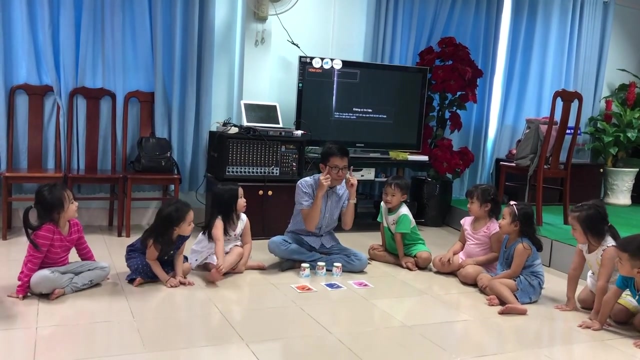 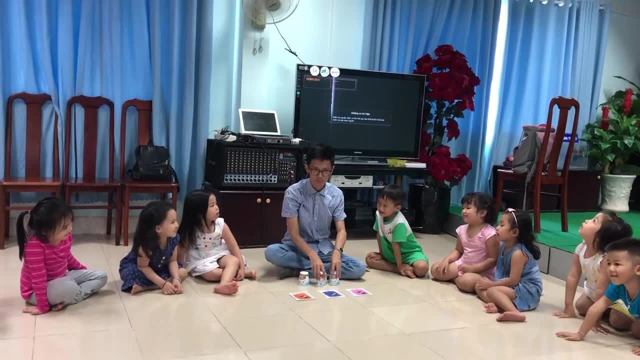 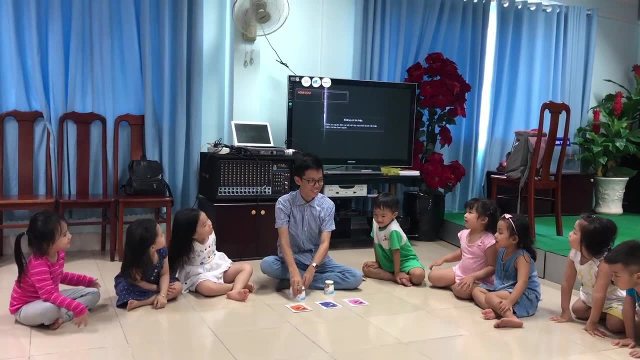 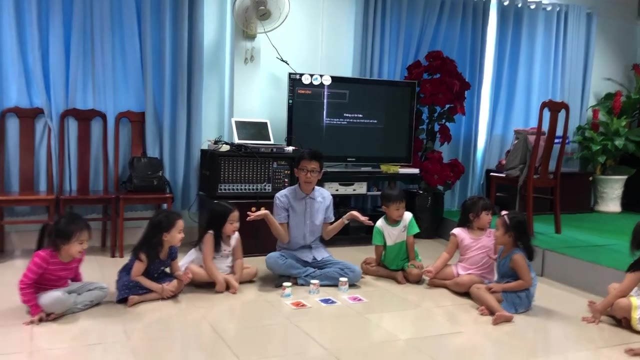 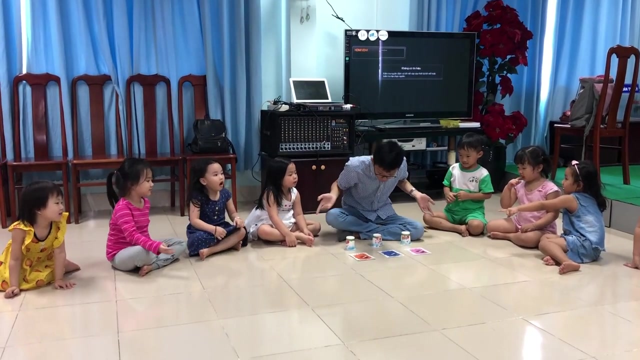 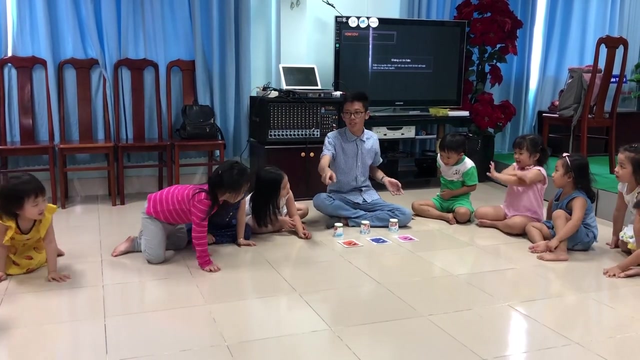 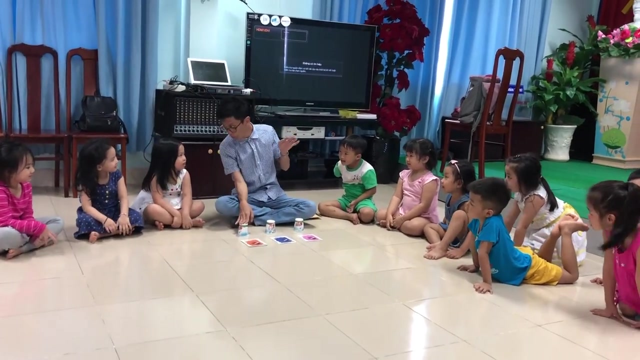 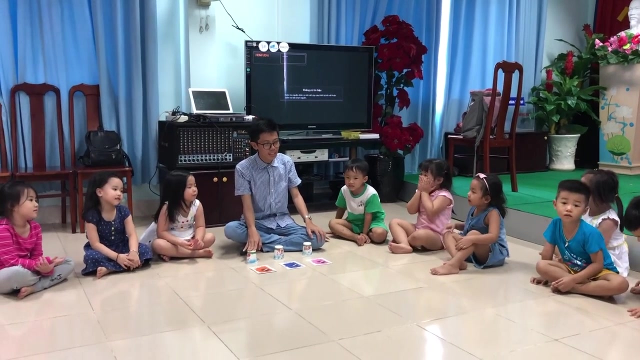 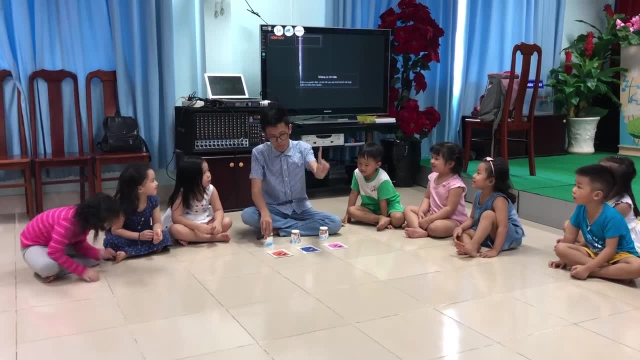 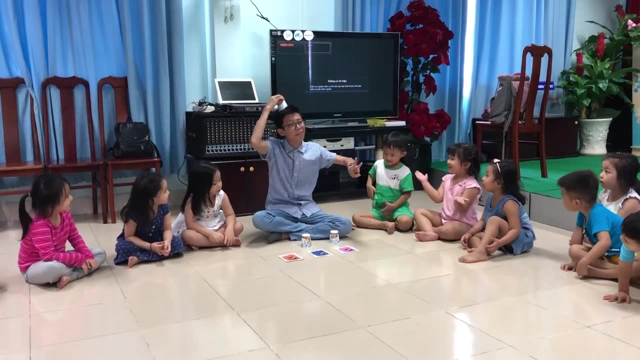 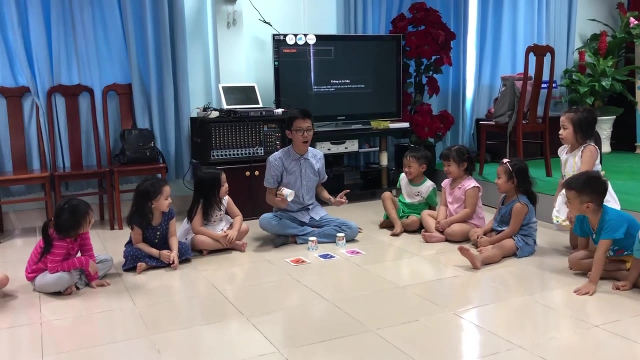 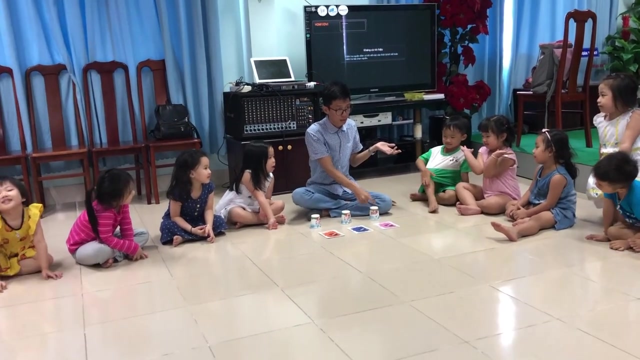 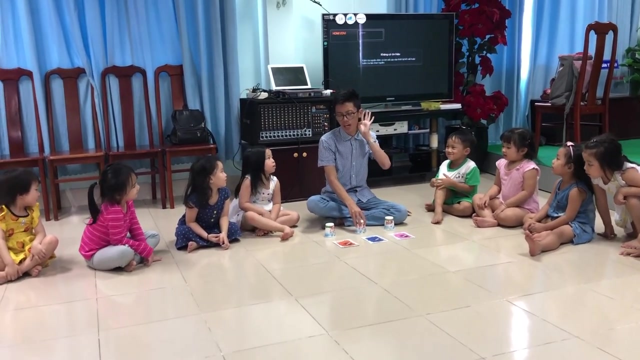 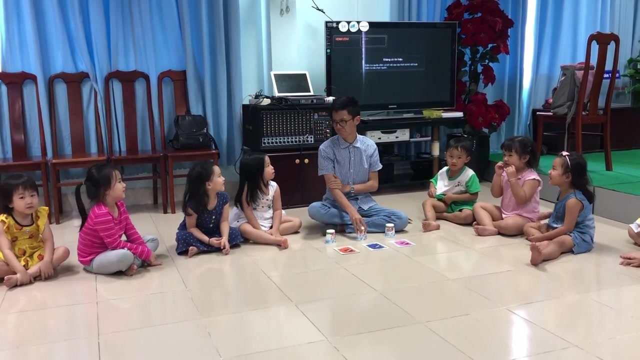 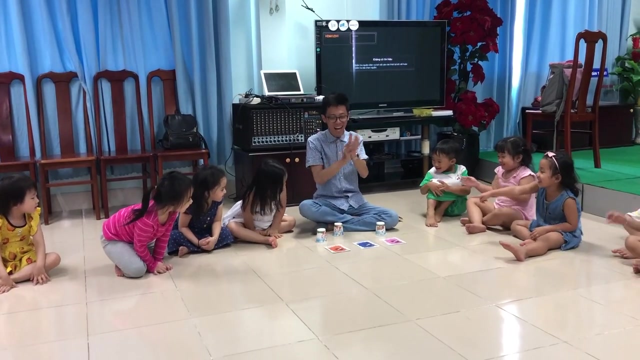 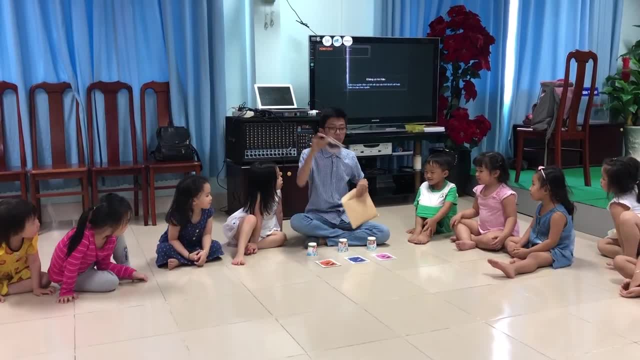 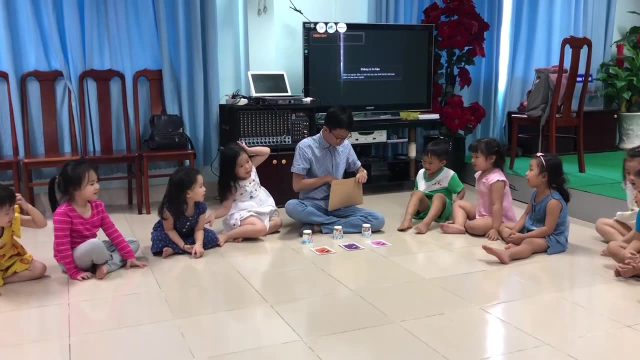 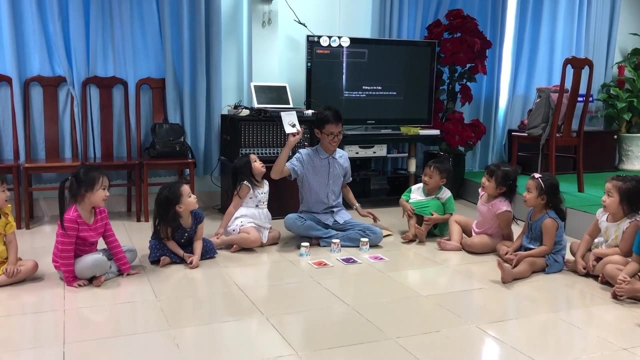 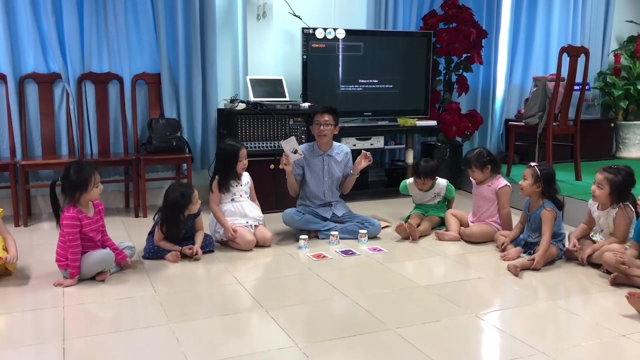 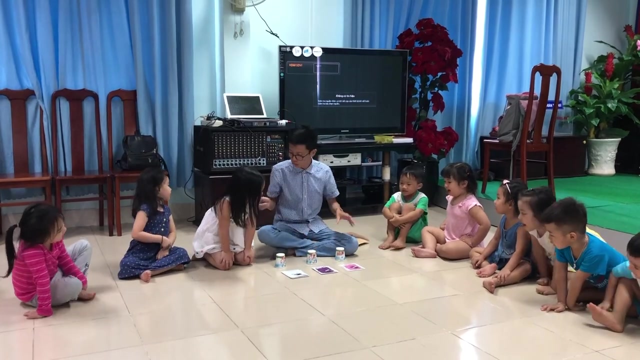 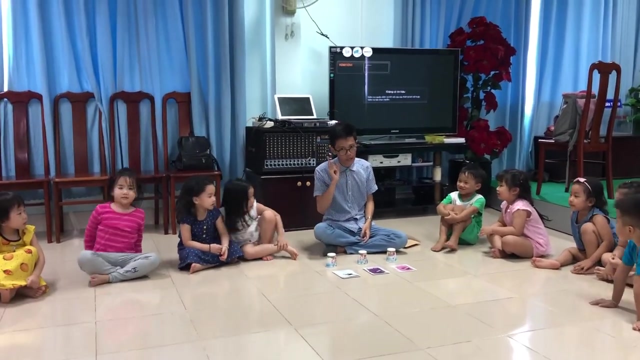 It's Blue. What color is it? It's Purple, It's Purple. What color is it? It's White. It's White, It's White, White, It's White. It's warm, Ready. Sit properly, Don't be so excited. Sit properly Like that. It's not proper. 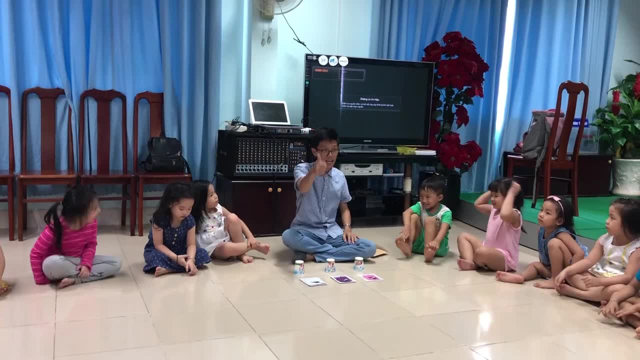 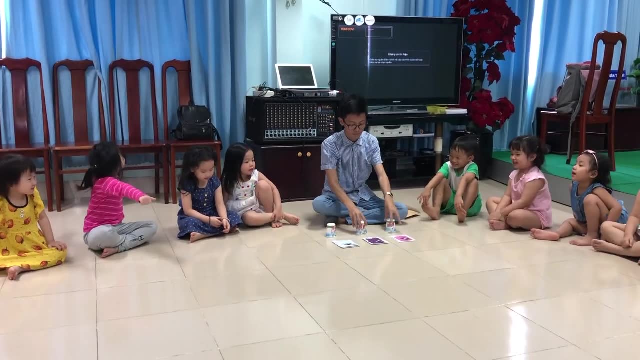 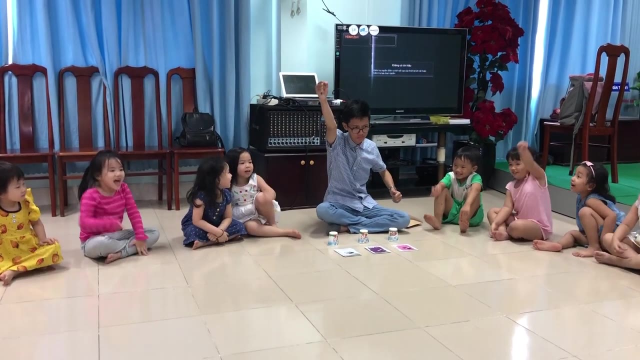 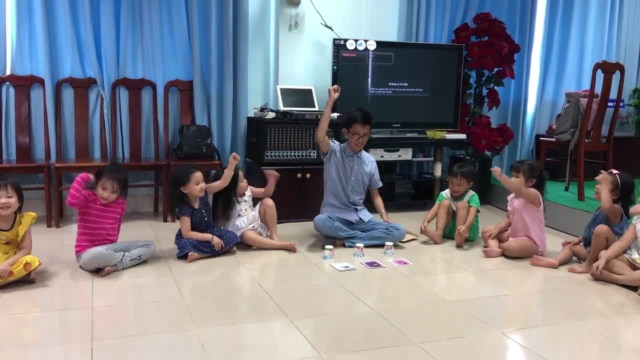 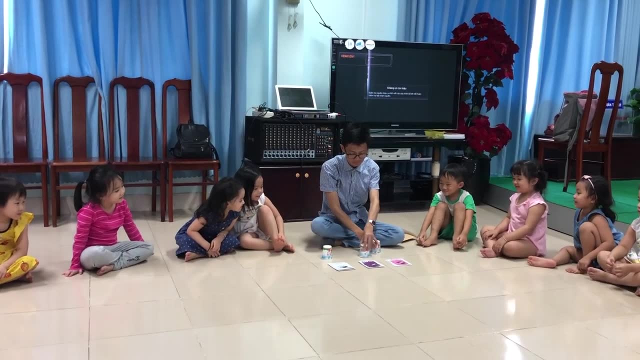 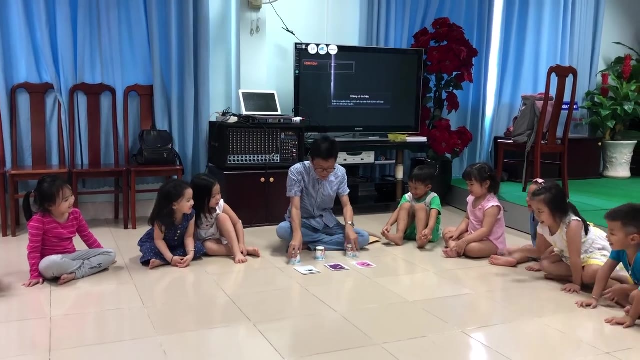 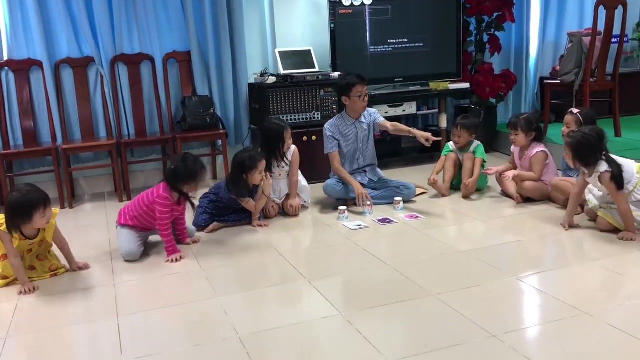 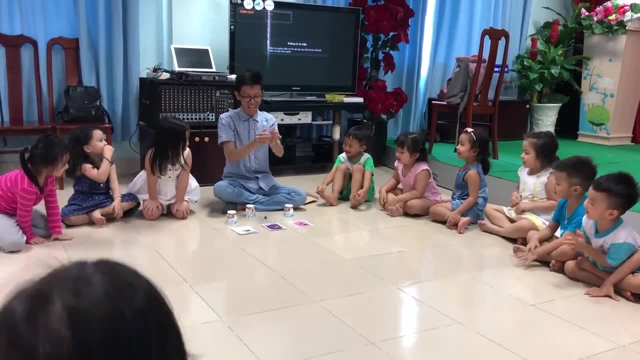 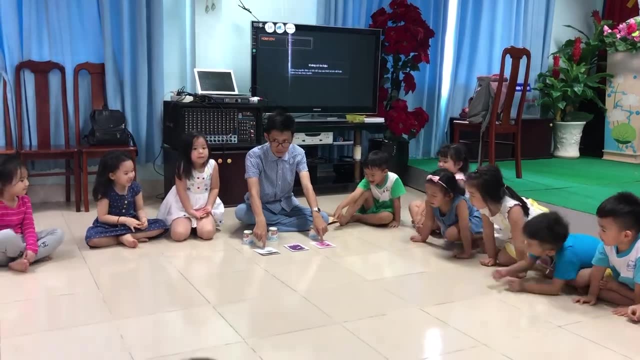 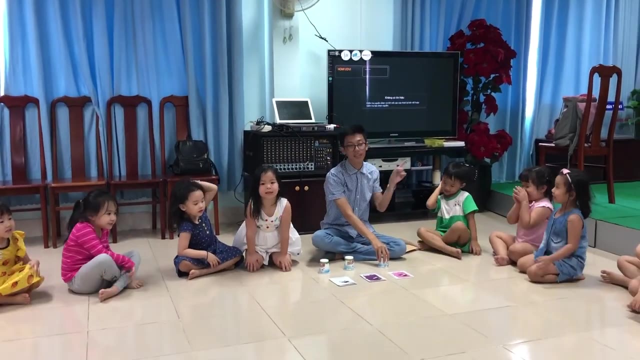 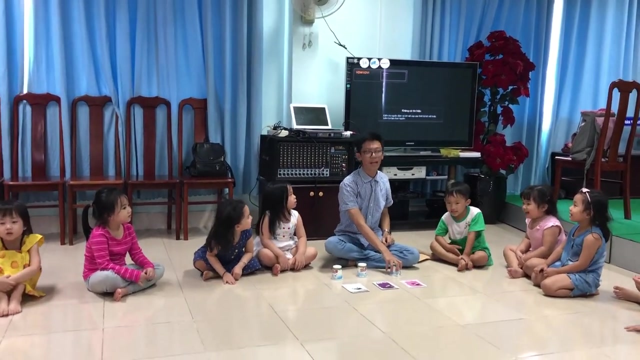 One, two, three go, Wow, Again, again, again Pink, pink, pink Where White or pink, White, White or pink, White, It's pink, It's pink. Again White, White, It's pink. 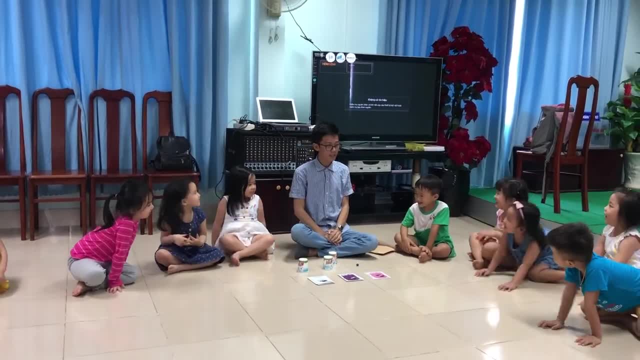 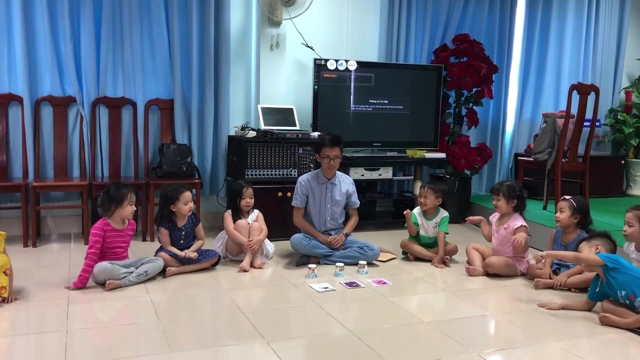 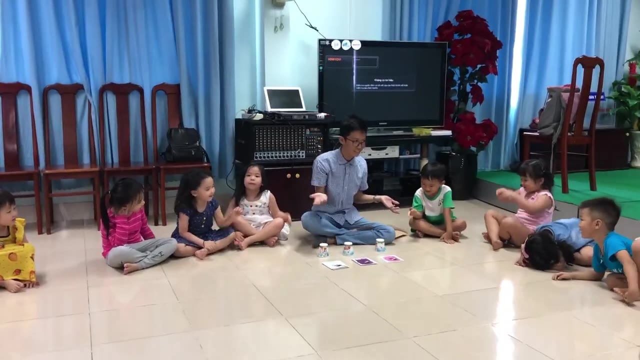 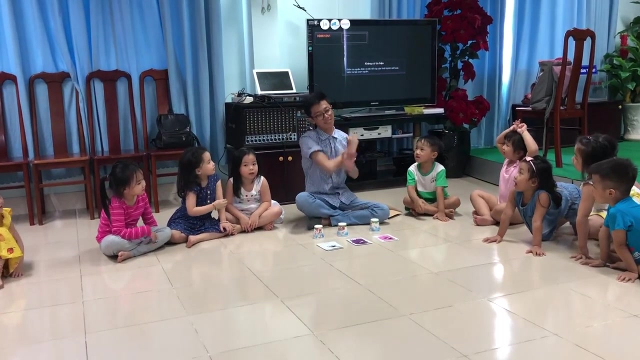 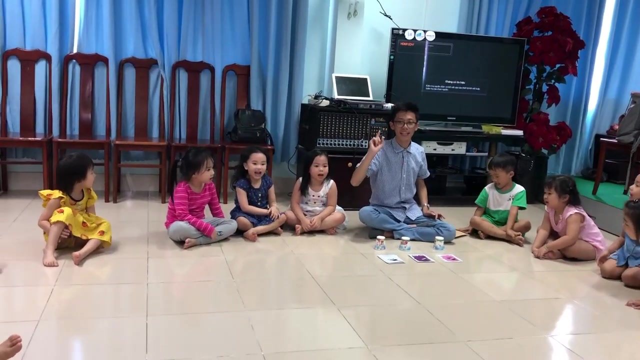 White, It's pink White, It's pink White, White, White. Oh Okay, where White White, White, It's white, It's white, It's white, I like white, I like white, I like white. 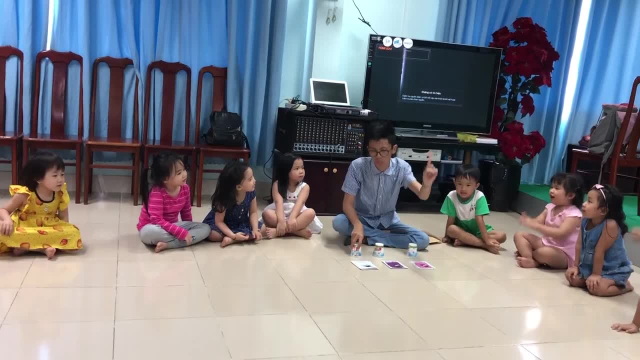 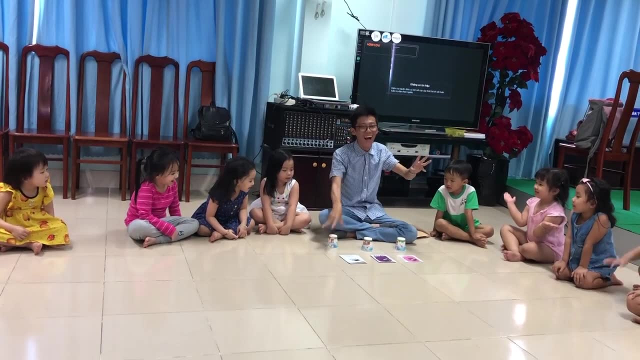 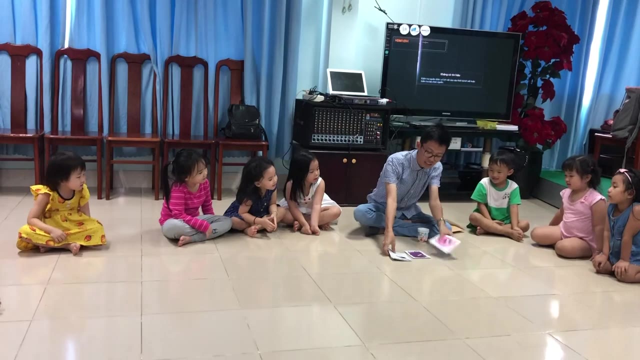 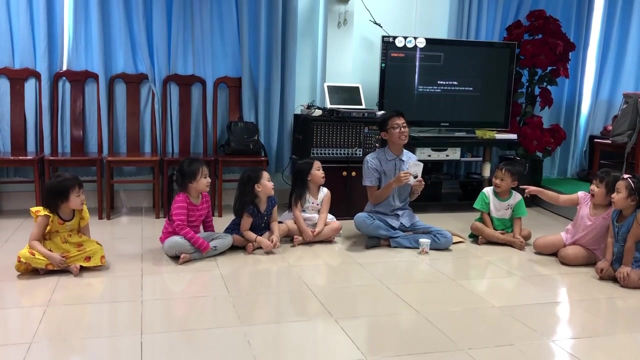 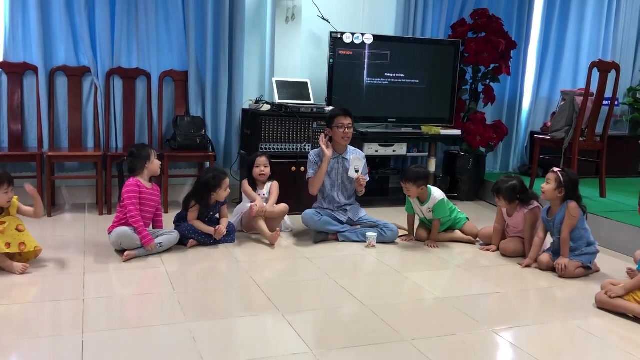 Let's go One, Two, One, Two, Three, Wow, Very good, Okay, let's review. let's review. Let's see if you know the colors. What color is it? It's white. It's white.